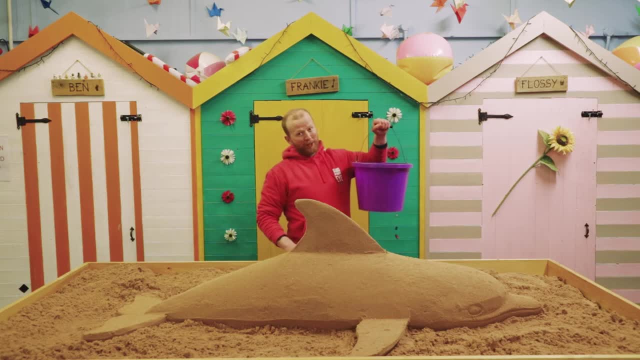 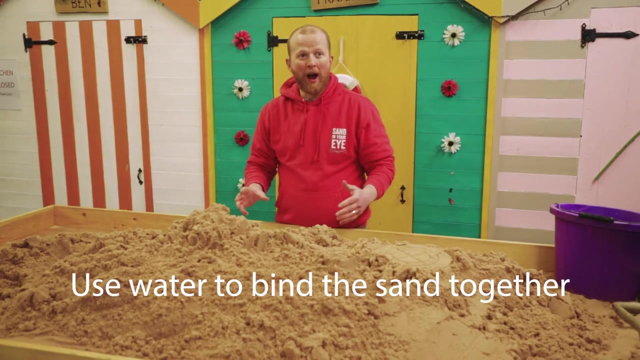 your sand with. you may need a bucket to collect all your water, with a wooden floor to carve, with a wooden spatula to do some sculpting and also maybe a lollipop stick just to do your details as well. If on a beach, you need to have damp sand now, you can do that by 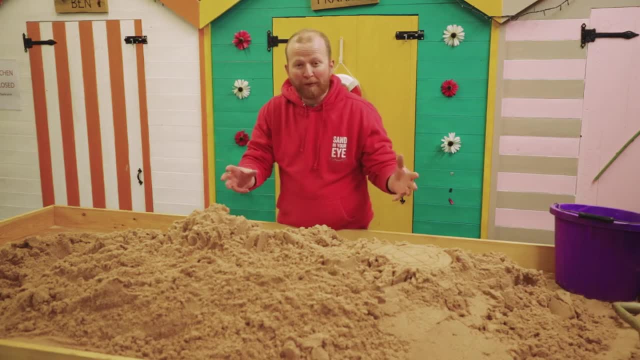 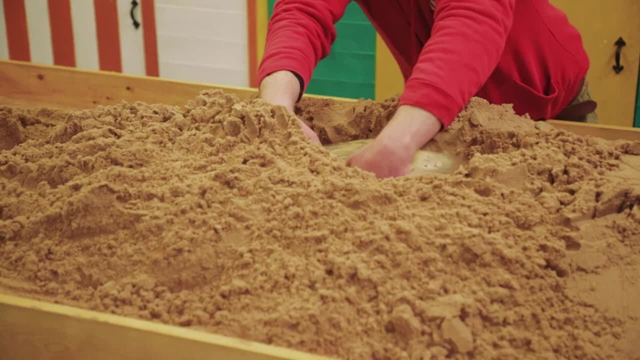 getting the sand below the high tide mark. you can get water from the sea using your buckets or you can even dig a hole. If your sand is dry, you can mix in some water. So, firstly, you make a rough shape of the dolphin, you get the sand and you push it together. 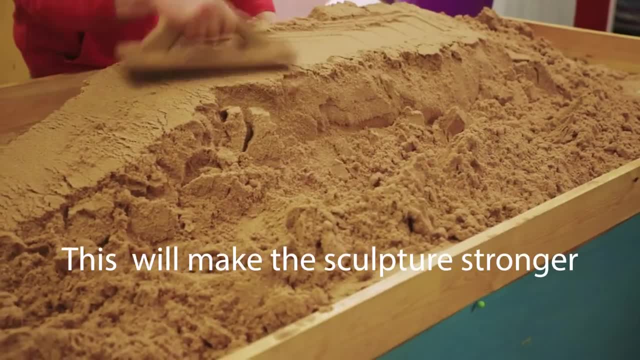 with your hands. So when we're making a sand sculpture, we have to make sure that the sand is completely dry. So we're going to make a rough shape of the dolphin. you get the sand and you push it together with your hands. So when we're making a rough shape of the dolphin, you get the sand and you push it together with your hands. So when we're making a rough shape of the dolphin, you get the sand and you push it together with your hands. So in this case, we're going to make a dorsal. 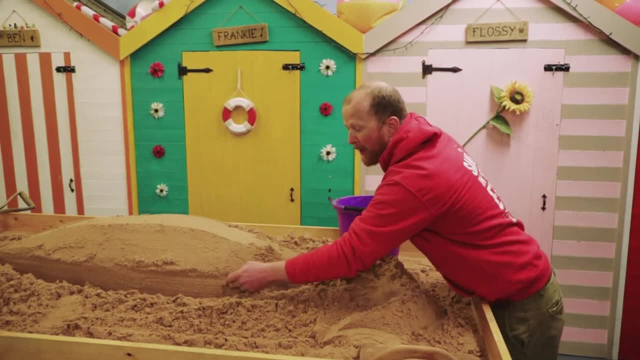 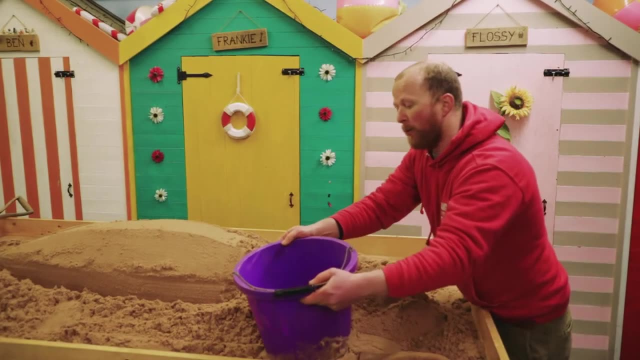 fin first. The reason is, if we make a pretty little eye like so, then when you're carving, all of the sand that will be on the top it's going to fall on it. So to make a dorsal fin we have to make mudpads or hand stacking To do this. we're going to get a load of sand. 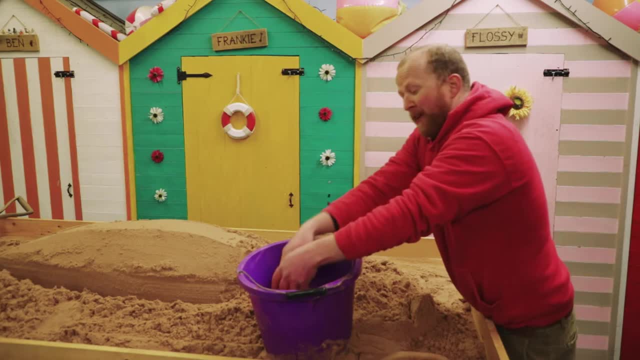 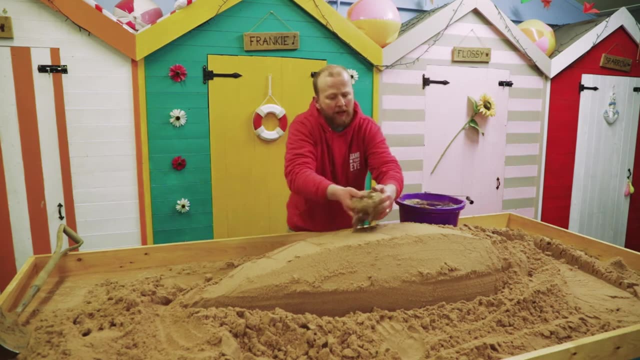 and we're going to put it into the bucket of water and fill it up, and the water needs to be above the sand. So to make a hand stack, we're going to take a load of really wet, sand it with one hand and then pat it with the other. Now it's really important to stop. 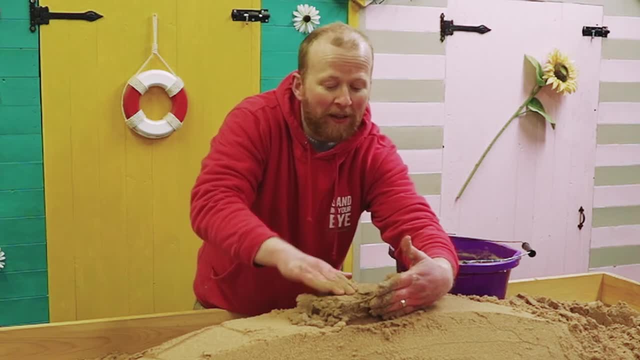 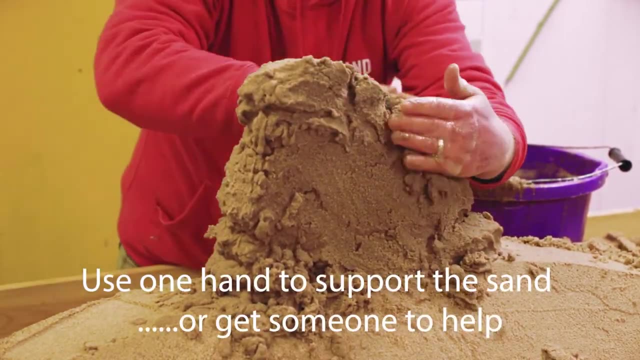 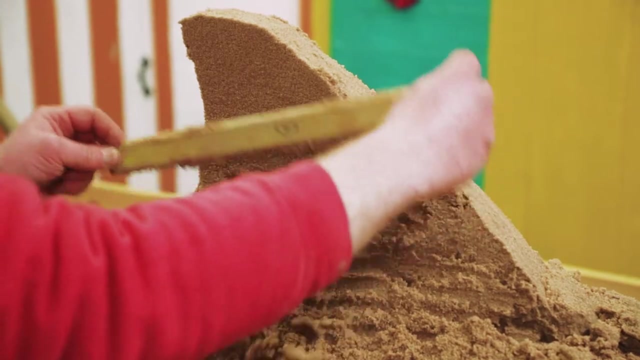 patting once the sand has set, else if we keep patting it actually just breaks it Gradually. stack up your mud pies in the shape of and a little bit bigger than the parcel of it, Then use a wooden spatula to cut your fin shape on the front and then the back and then 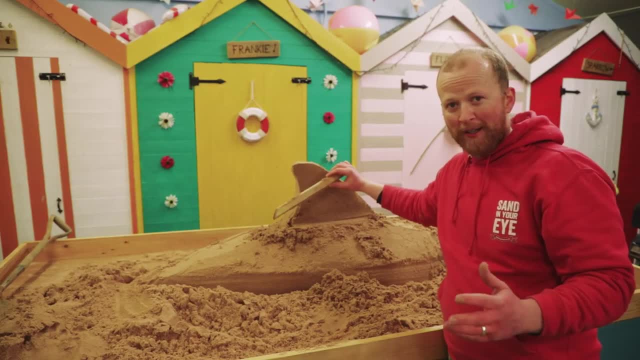 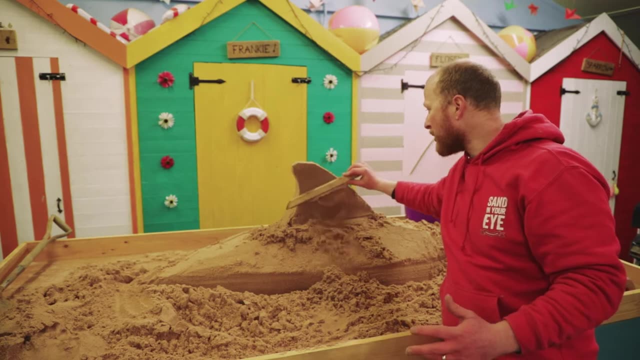 cut off the sides. So if there's one thing with sculpture that I can tell you is when you are doing, your cuts always cut into the body of the sculpture. So I'm trimming the dorsal fin off this way, because if you cut the other way, then this is what happens. 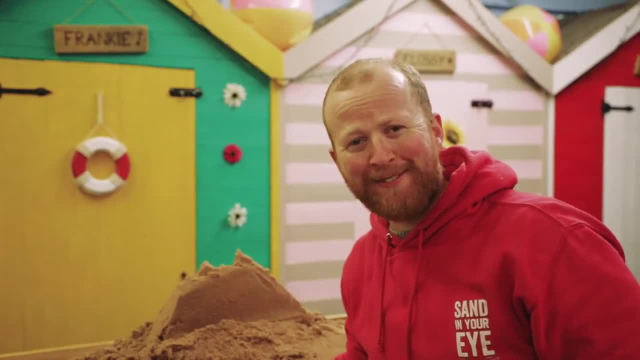 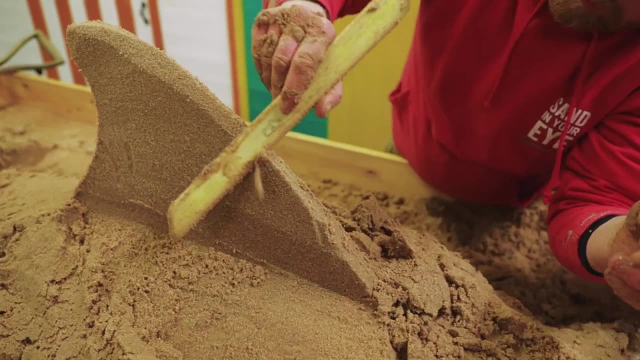 Why did I do that? Now I'm gonna have to start all over again. Then we'll sketch a centre line and then cut it off so it's nice and tapered and streamlined, whilst keeping the dorsal fin a little bit thick so that it's nice and straight. So once you've